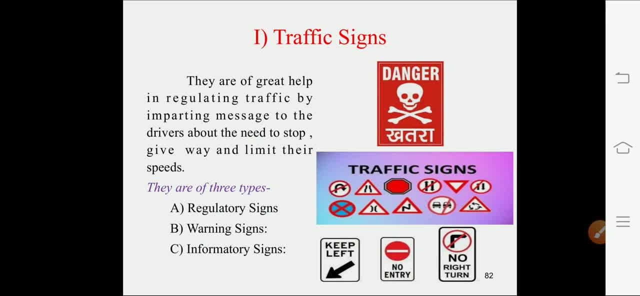 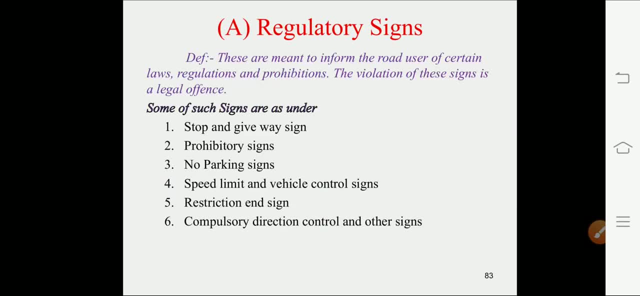 Okay, So all that are categorized in this several types, that is, regulatory, warning and informatory signs. So what is this? regulatory signs: These are meant to inform the road users of certain laws, rules, regulations and prohibitations. The violation of these signs is a legal offense. 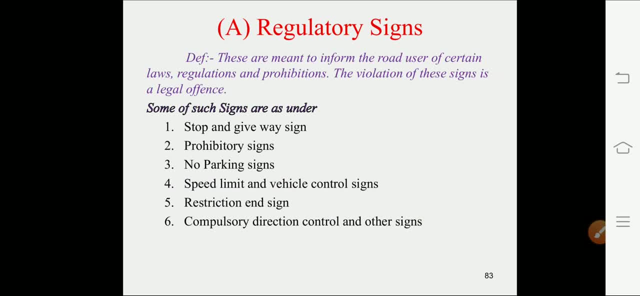 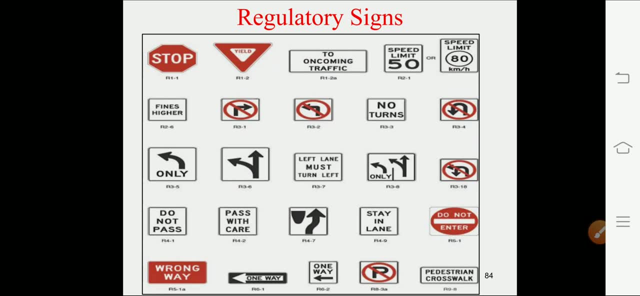 Some of such signs are as under: stop and give way sign. Okay, Stop and give way sign. Many a times you might have studied all these types. You might have seen all these types of sign: boards, prohibitory signs, no parking signs. 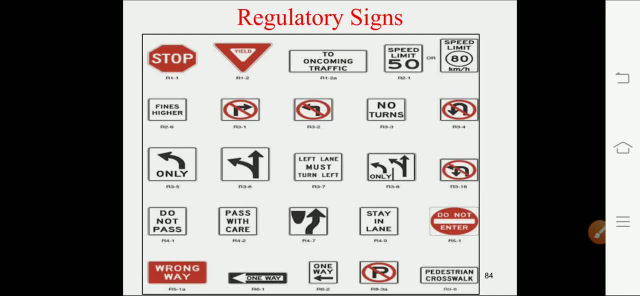 Okay, So right turn prohibited. left turn prohibited. no turn, only one side turn. Okay, Wrong way. do not enter means, if it is a one way they are many times writing: do not enter. U-turn is restricted Speed limits. they are giving you the banner of speed limit. 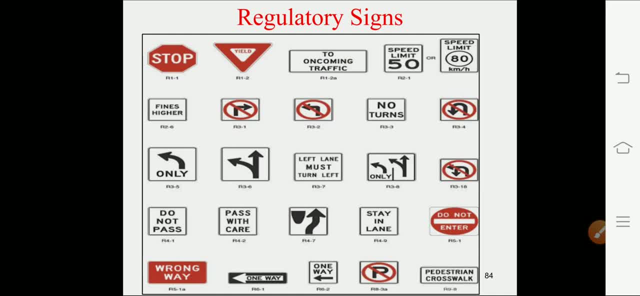 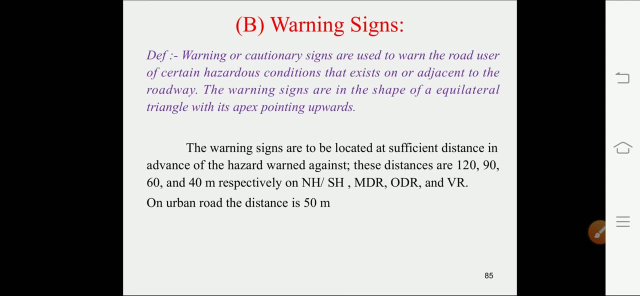 All these are the regulatory signs. You have to follow the rules. Okay, Then. restriction in signs, compulsory direction signs- Okay, Then all these are regulatory signs. Next is warning signs. What are the warning signs then? Warning or cautionary signs are used to warn the road users of certain hazardous condition that exist on or adjacent to the roadway. 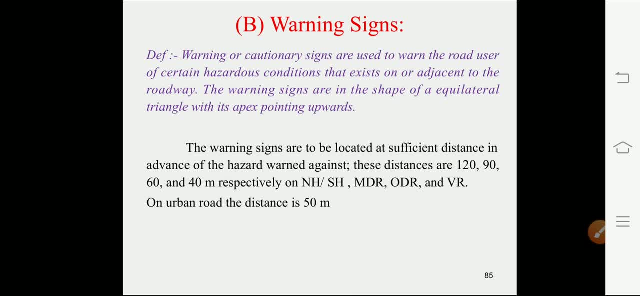 The warning signs are in the shape of the equilateral triangle and it's apex pointing upward. The warning signs are to be looked at. The warning signs are to be located at sufficient distance in the advance of the hazardous one against. the distances are 120, 90, 60, 40 respectively on national or state highway, major district road, other district road and village road. 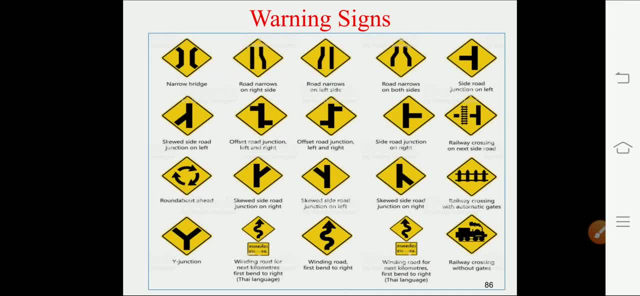 On urban roads. the distance is 50 meters. So such type of warning signs- it is in shape with apex at the top, Okay, So this type of again signs, many a times you might have come across, showing you there is a narrow bridge: road narrowed at right side, road narrowed on left side, road narrowed on both the sides. 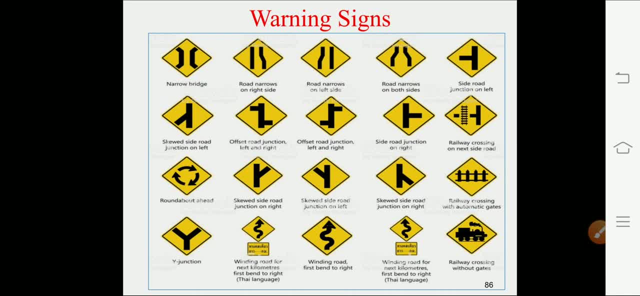 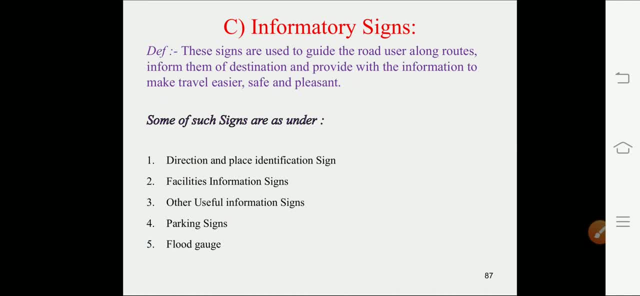 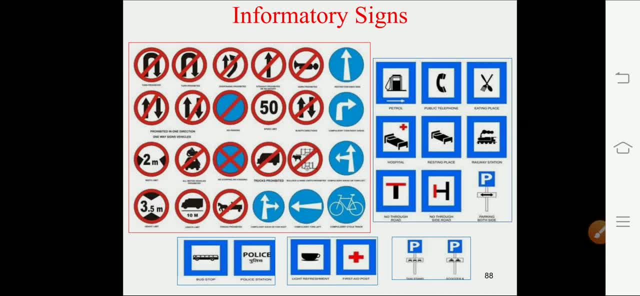 Then some of the signs are of this kind of informatory signs Many a times. if there is a hospital, it will show the symbol of hospital, like bed and plus sign. Then if there is a hotel, they will show you the spoons, okay. then if there is a parking facility, it will be, uh, noted with a p and two. 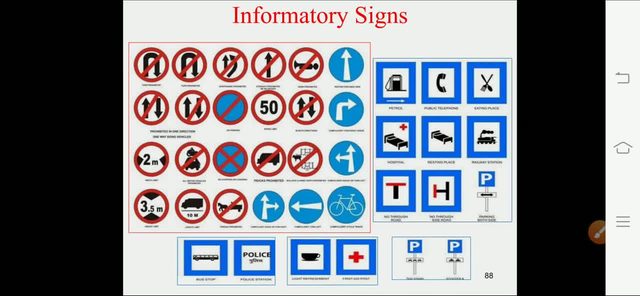 wheeler and four wheeler symbols will be denoted if there is a railway station ahead. likewise, railway will be shown again. informatory signs will also be, uh like if u-turn is probably prohibited, and all all such types of information they are giving you, like parking signs, flood gauge. 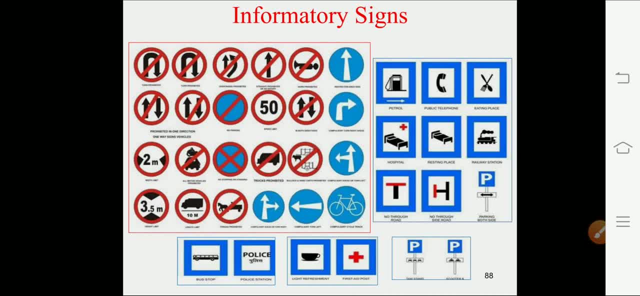 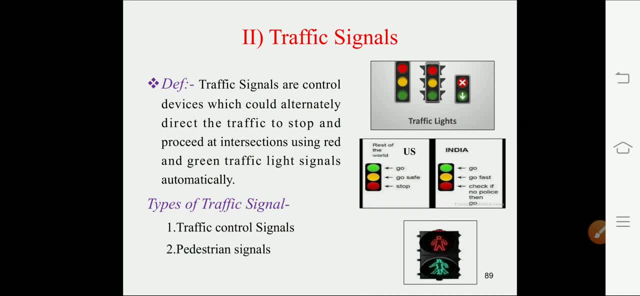 facility is information, size, etc. then traffic signals: many a times in cities when we go we come across the signals, whereas this is not possible in our local towns. this helps to properly regulate the traffic. traffic signals are control devices which contains alternate only direct. alternatively, direct the traffic to stop and proceed at intersections using 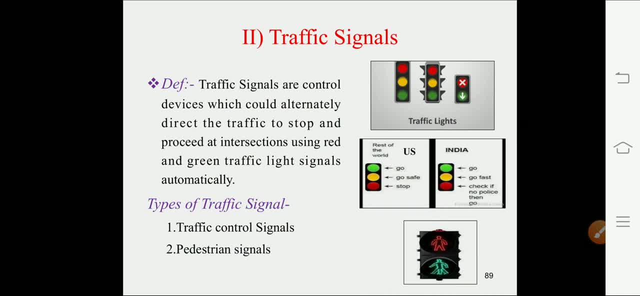 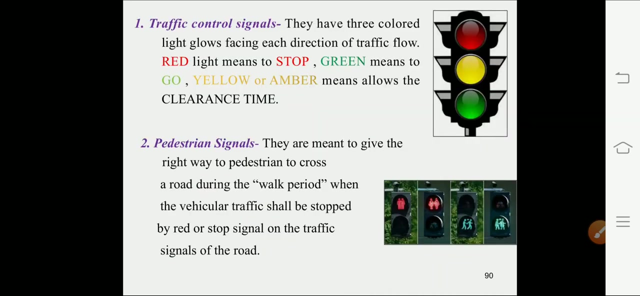 red green light traffic lights signals- atomic, automatically- okay, types of traffic signals, traffic control signals and pedestrian signals: okay, for those who are walking, for them also, signals are provided and for vehicles, as usual it is also provided. so traffic control signals. they have three colors here in figure also you can see. 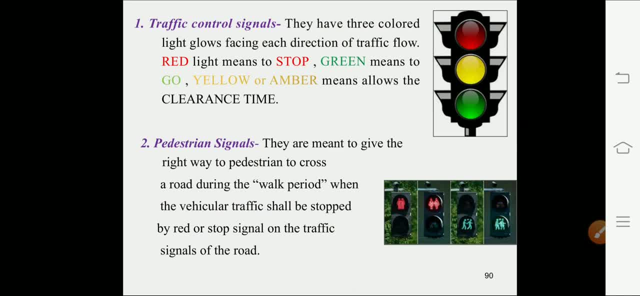 light glows facing each direction of traffic flows. red light means stop, green indicates to go and yellow number means to. it is nothing but a clearance time and for pedestrian signals, that is, for the person who are walking. they are meant to give the right signal to the pedestrian to cross a road during the walk period, when the vehicular traffic should. 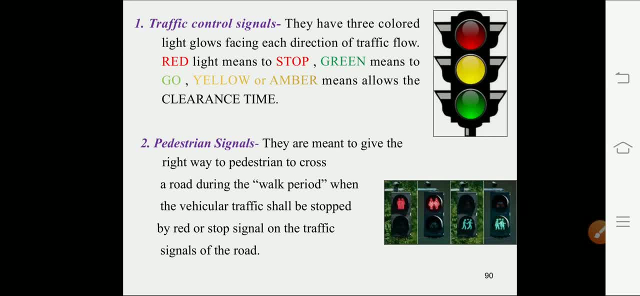 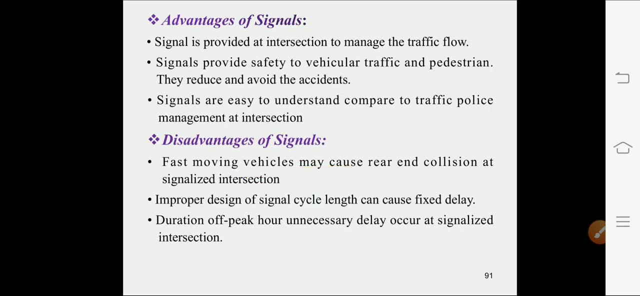 be stopped by red or stop signals on the traffic signs. if it is showing red, that person has to stop. if it is showing you green, then that person has to move over a for a walking period. advantages of these signals are: signal is provided at intersection to manage the traffic flow. 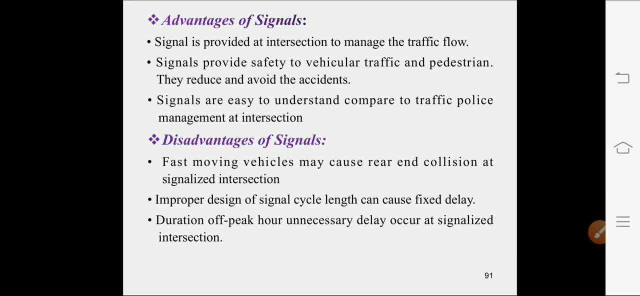 signals provide safety to vehicular traffic and pedestrians. they reduce and avoid the accidents. signals are easy to understand compared to traffic police management at intersections. there are also some disadvantages of these signals, like fast moving vehicles may cause rear rear end collision at signalized intersections. improper design of signal cycle length can cause fixed delay. 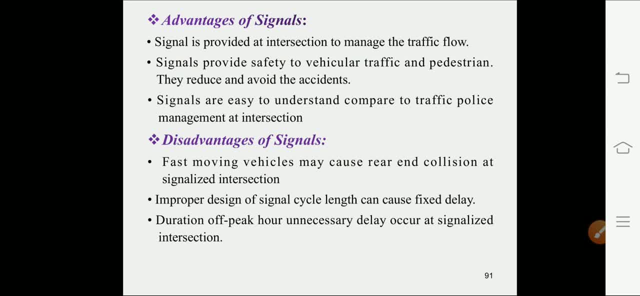 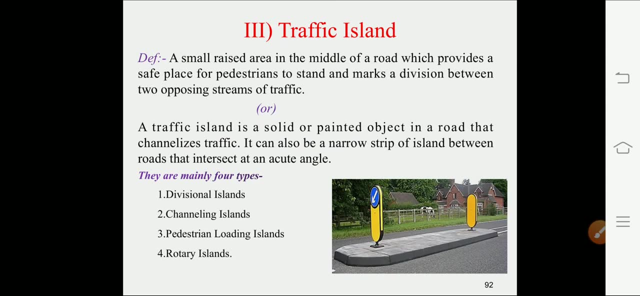 pick are unnecessarily delay occurs at signalized intersections. many a times you might have faced many problems at the signals. okay, then traffic islands. the figure first. see the figure. traffic island. this: this shows you the separators: a small raised area in the middle of the road which provides a safe place for pedestrians to stand and marks a division between two opposing streams. 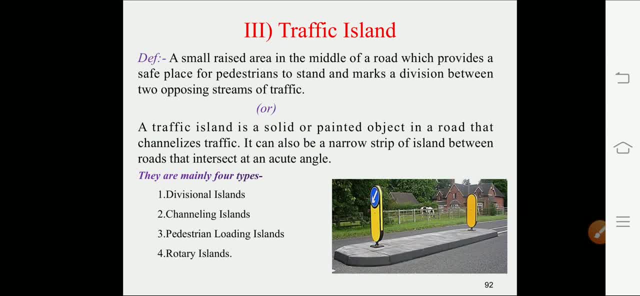 of a traffic is called as a traffic island. in other words, a traffic island is a solid or pented object in a road that channelizes traffic. it can also be narrow strip of island between the road that intersect at an acute angle. again, there are mainly four types of traffic island. 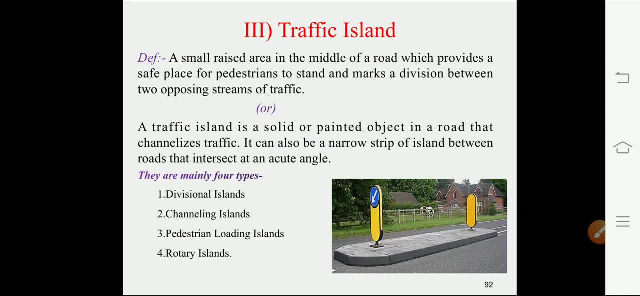 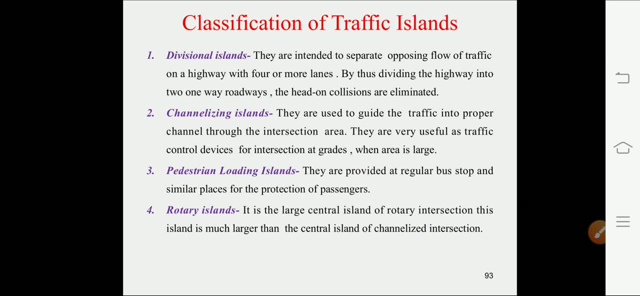 divisional island, channel island island, pedestrian loading island and rotary island. so what is divisional island? they are intended to separate opposing flow of traffic on a highway with four or less lanes by these dividing the highway into two or two, dividing two one way roadway, the head-on collisions are limited. 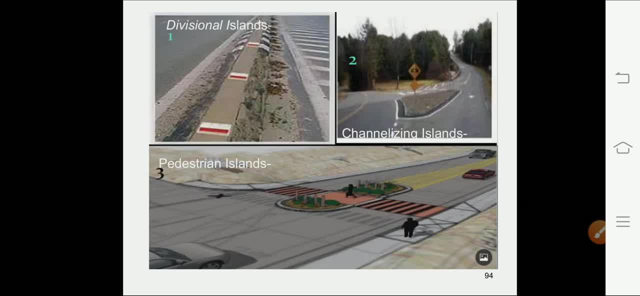 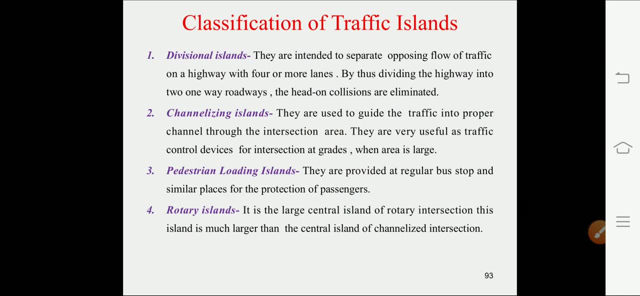 so see the first figure. these are nothing but the divisional island channelling islands. these are used to guide the traffic into proper channelling island. these are used to guide the traffic into proper channel through the intersection area. they are very useful as traffic control devices for intersections at grades when area is large. second figure: you can see two roads. 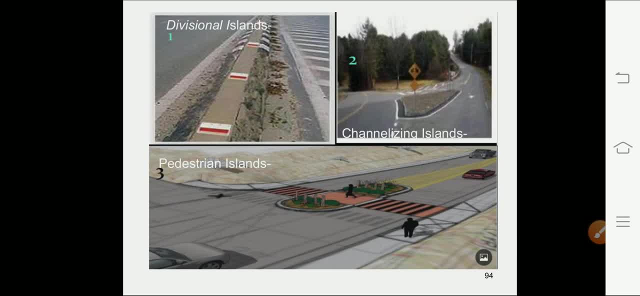 are passing, they are getting diverted from each other. so, whatever will be the middle portion, there, this portion is raised up to two. rated a middle portion. there, this portion is raised up to two, rated a, which is nothing but a channelizing island. this helps to segregate simply. 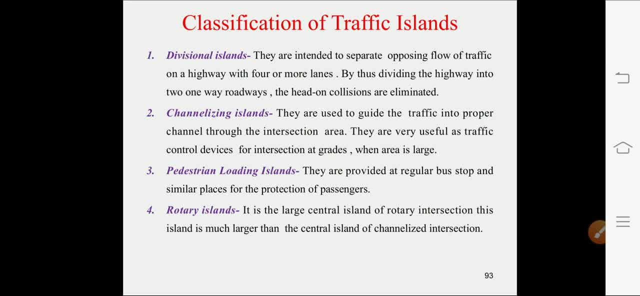 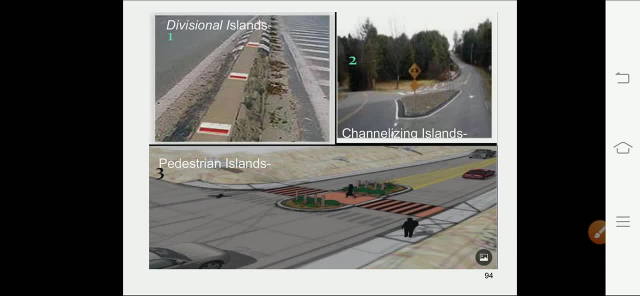 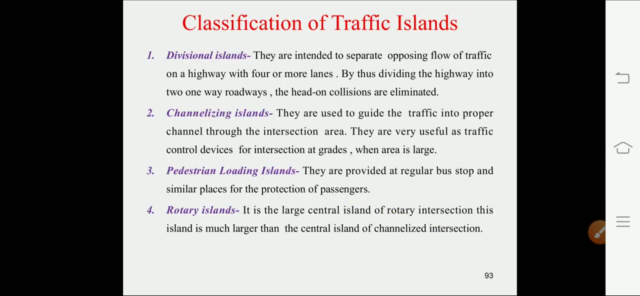 then pedestrian loading island. these are provided at regular bus stops and similar places for the protection of passengers. so here, pedestrian islands. third one, you can see the middle portion is quite raised so that the walkway for the person's walking through are been taken due care, and a rotary island it is. 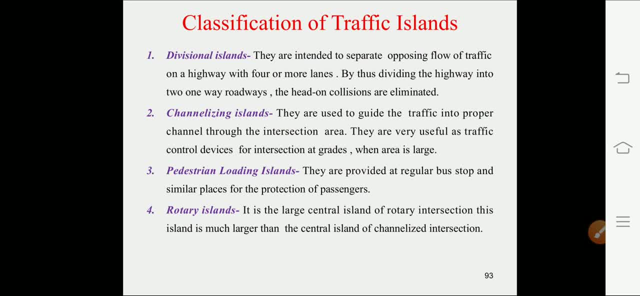 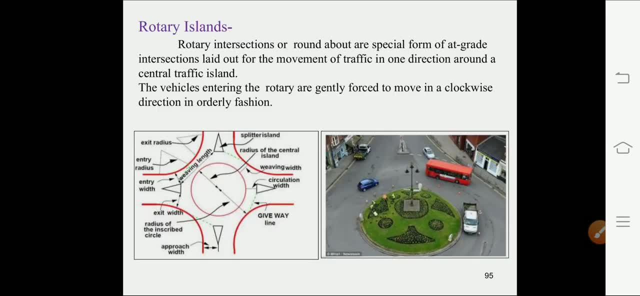 the large central island of rotary intersection. this island is much larger than the central island of the channelized intersection. this is the rotary island. this is also called as a roundabout. these are the special forms of at grade intersections laid out for the moment of traffic in one direction. 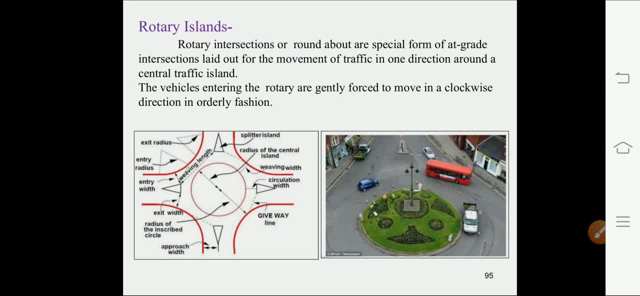 or the central traffic island. okay, now see, like this: roundabouts, are there the vehicle? if you it have to take turn, it have to all round move around this roundabout, then it have to take. this helps to eventually reduce the accidents: head-on collisions. the vehicles entering the rotary are generally forced to move. 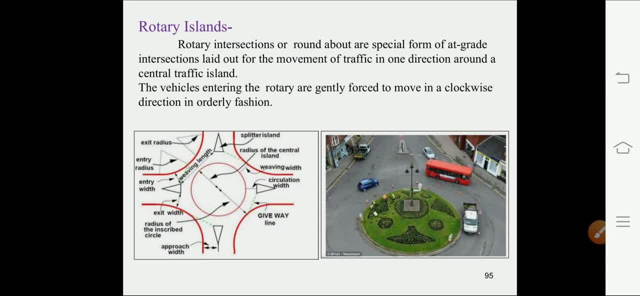 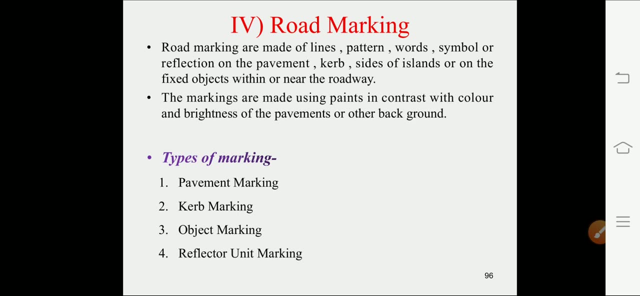 in the clockwise direction in orderly fashion. okay, so generally along the roundabout you have to always move in a clockwise direction. lastly, road marking. road markings are made of lines, patterns, words, symbol or a reflection on the pavement, curbs, side of island or on the fixed object within or near the roadway. 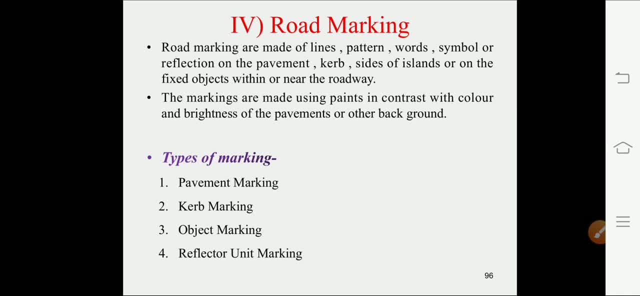 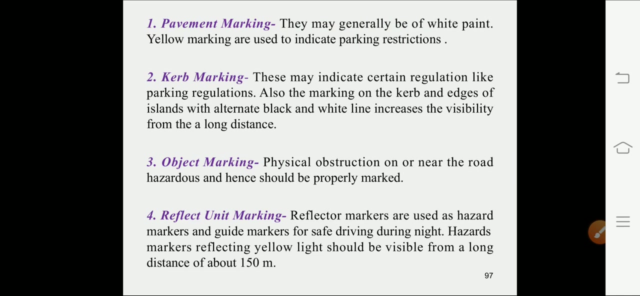 the markings are made using pens in contrast with color and brightness of the pavements or other backgrounds. there are several types of marking, like pavements marking, curb, parking curb marking, object marking, reflector, unit marking. then what his pavement marking they are generally have painted with white color. yellow marking are used to 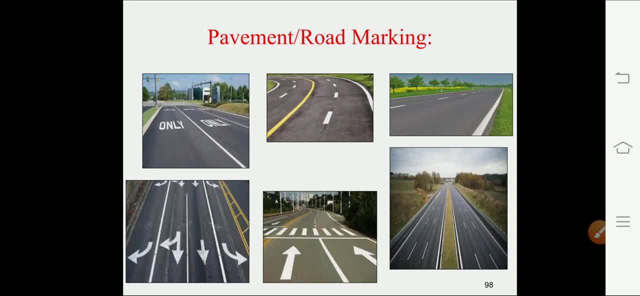 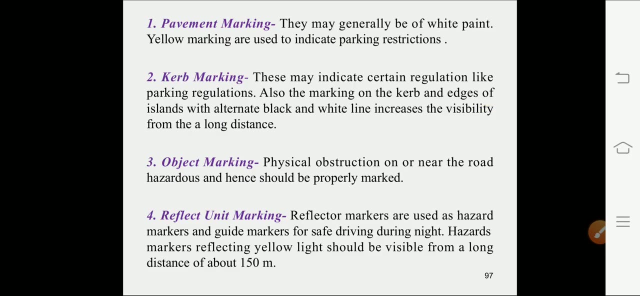 indicate parking restrictions. ok, so this, this type, ok, like this many a times you might have seen also: white it gives you the indication for the movement, whereas red it is the restricted area curve marking. these are indicate this. this may indicate certain regulations like parking regulations. also, the marking on the 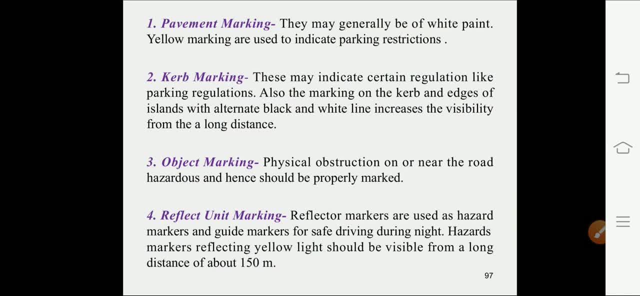 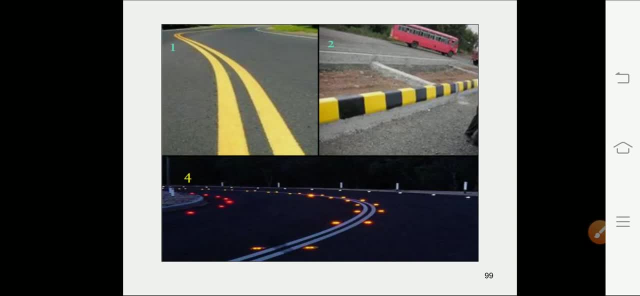 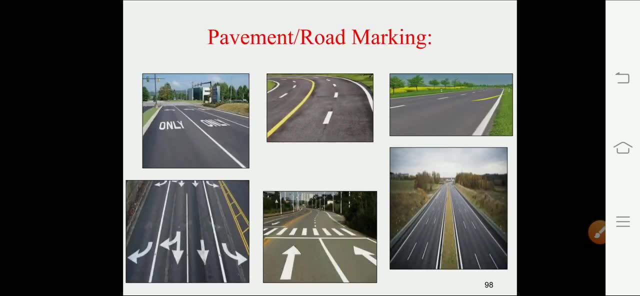 curve and edges of the island with alternate black and white lines increase the visibility from the long distance. so here, like this curve raised portion by this, what happens from the long itself, we can see that there is a curve marking object, marking physical obstructions on or near. 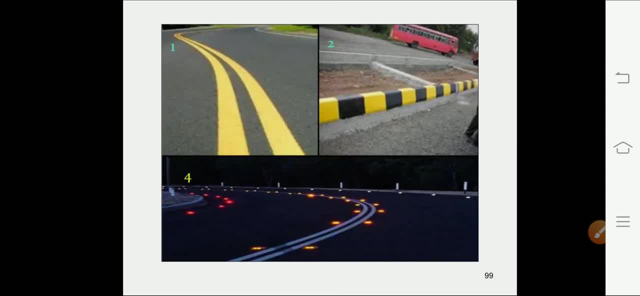 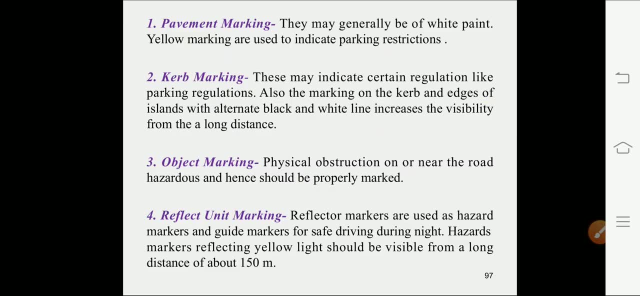 the road hazards and hence it should be properly marked. okay, if there is any object, it should be properly marked, otherwise it will get damaged and reflect unit marking. reflector mark markers are used as hazardous markers and guide markers for safe driving during night. many times, if you move along the expressways, you see the blinking of radium. right, it is nothing. 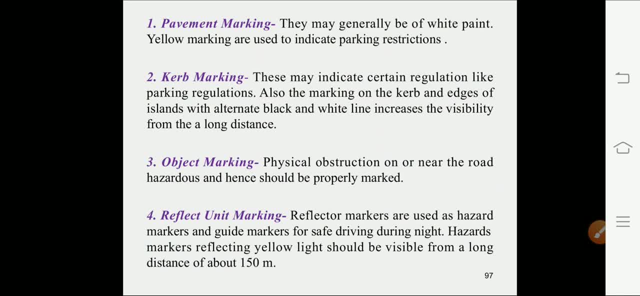 but reflecting light. it is nothing but the reflection of light. when was the light falls on that? it's? it blinks or it reflects the light. it helps to properly guide the driver about the turning hazards. hazards mark markers reflecting yellow light should be visible after a long